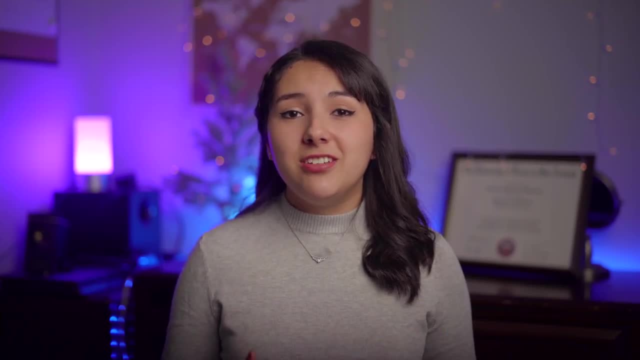 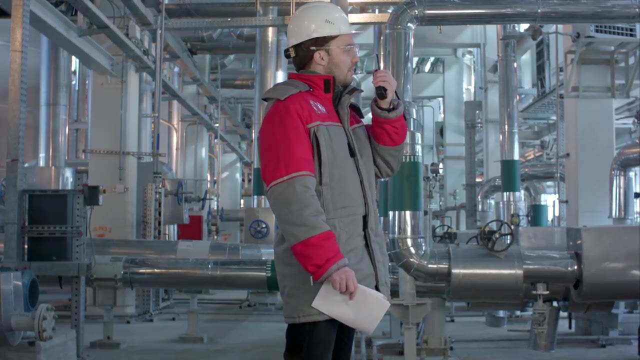 biology. So what are some of the things you should be interested in learning about in your career? biology. A lot of your classes will use engineering principles applied to biological systems. So, for example, instead of having to find the volumetric flow rate in a pipeline, you will be using similar. 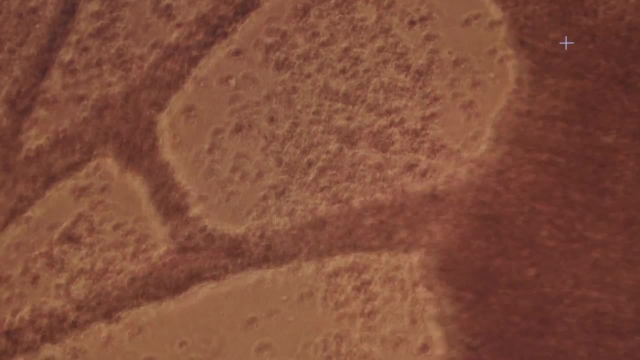 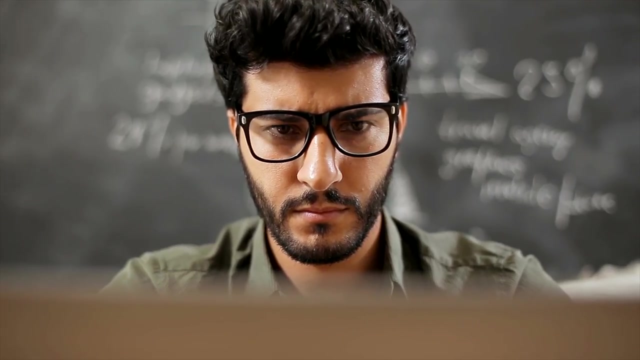 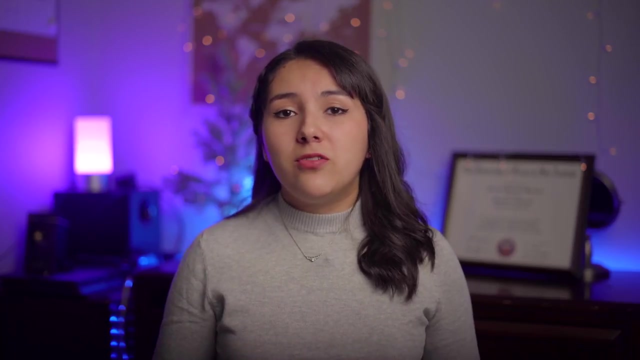 principles to study flow rate through blood vessels. Number two: you enjoy solving problems and using critical thinking. The core of an engineering degree is the ability to solve problems and think critically. This is no different for biomedical engineers. In a biomedical engineering degree, most of your classes will have some memorizing to do when it comes to biology. 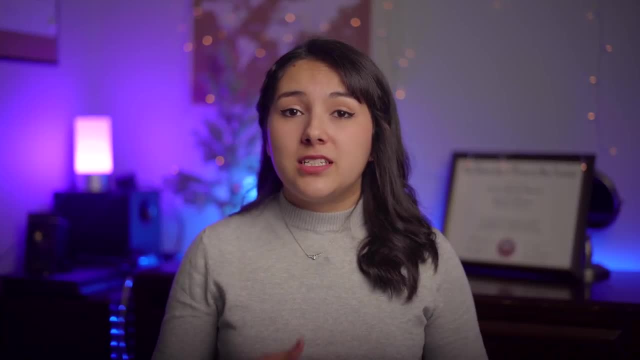 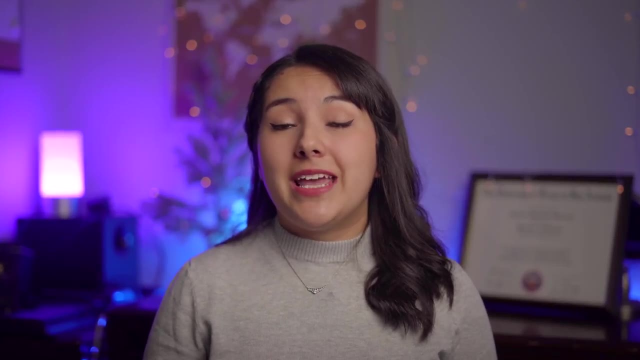 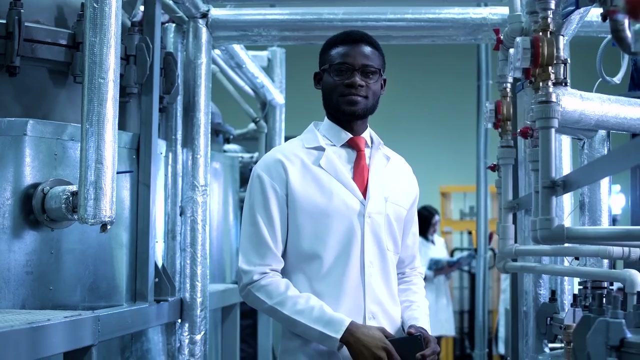 and medical terminology, But most of your classes will develop you as a researcher, engineer and scientist. Your ability to solve problems and think critically will be exercised every single day. Number three: you have a desire to improve the world, Specifically in the field of human health. you might have noticed that the last two reasons could 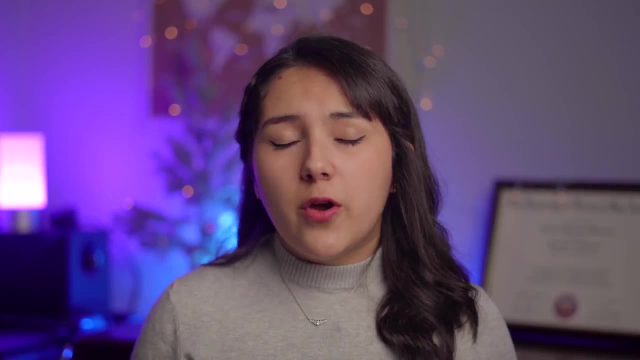 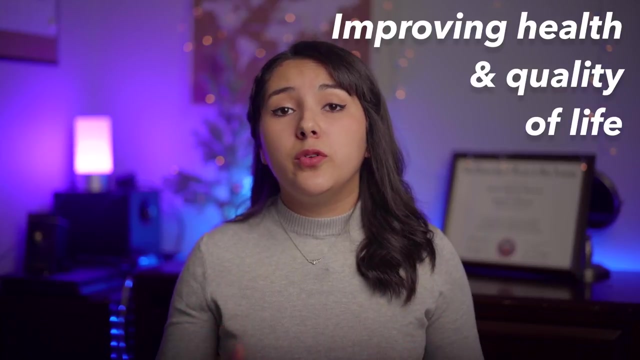 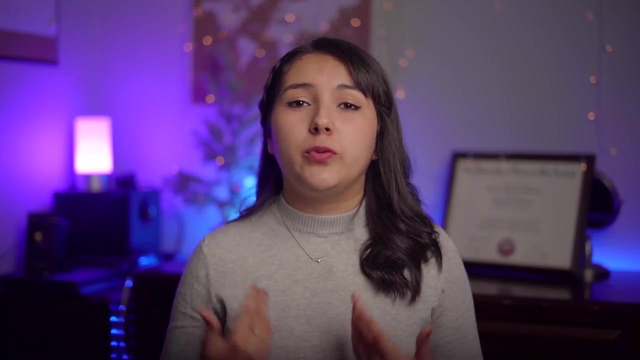 apply to any engineering degree, Then why should you focus in biomedical engineering? Well, if you want to use the engineering knowledge to specifically study and improve human health, then BME is for you. Most BMEs choose the field because they have a personal passion to improve. 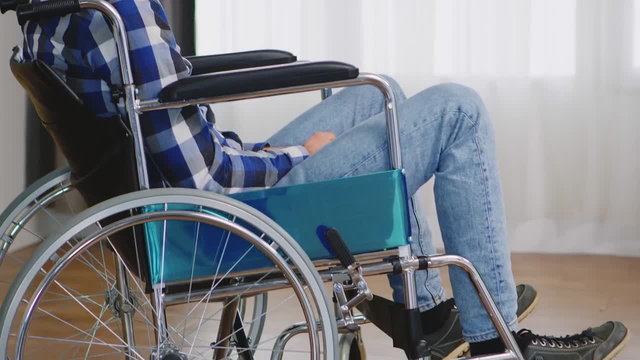 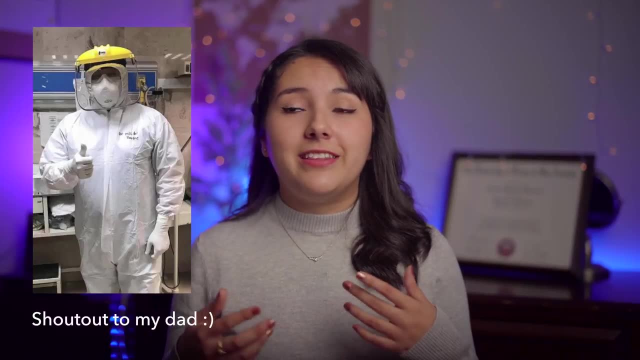 someone's health. Some BMEs have personal battles with medical conditions or have a loved one who does. Others have family members who are healthcare professionals and thus they're interested in the healthcare field, Whatever the source is, even if it's just because you think BME sounds cool. 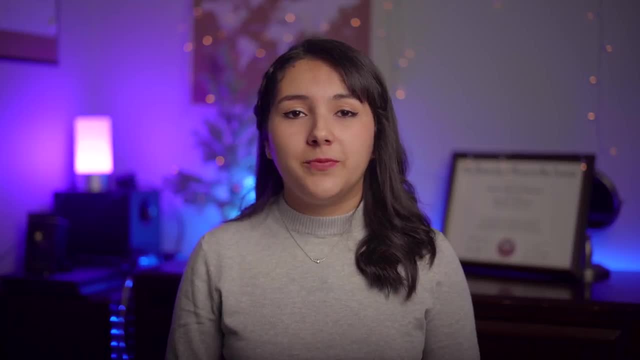 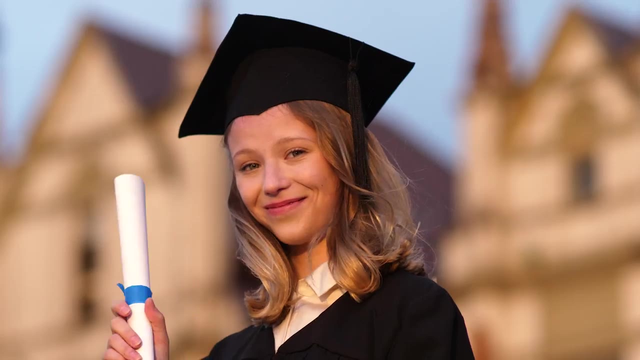 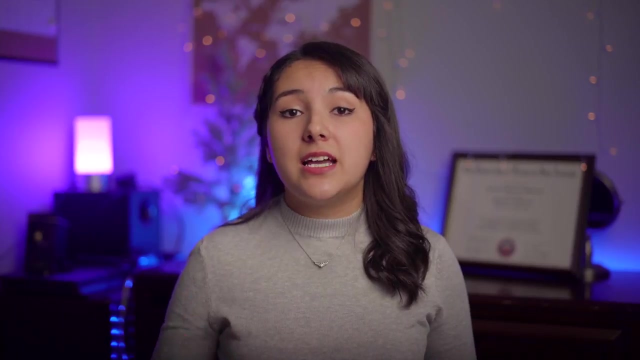 BMEs want to make a difference in human health. Number four: BME gives you the opportunity to study up to any level of education, whether it is a bachelor's, a master's or a PhD. You don't need a master's or a PhD to be a successful biomedical engineer. You don't need a master's or a PhD to be a successful 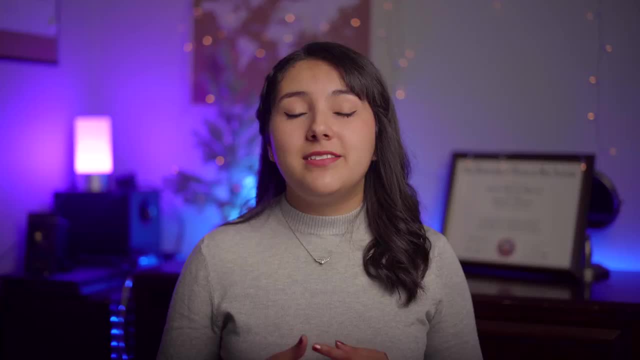 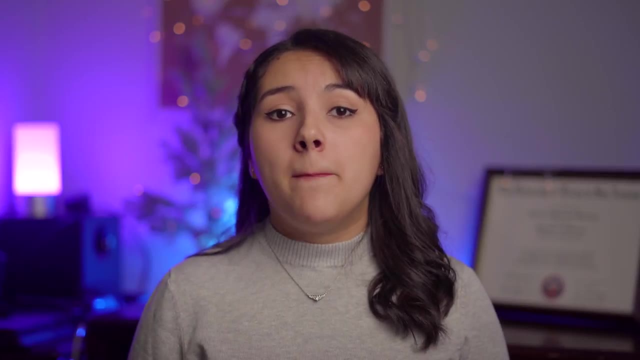 biomedical engineer. You don't need a master's or a PhD to be a successful biomedical engineer. In fact, most BMEs study up to a bachelor's degree. However, doing a master's or a PhD will definitely give you more specialized knowledge and make you a more competitive candidate when it 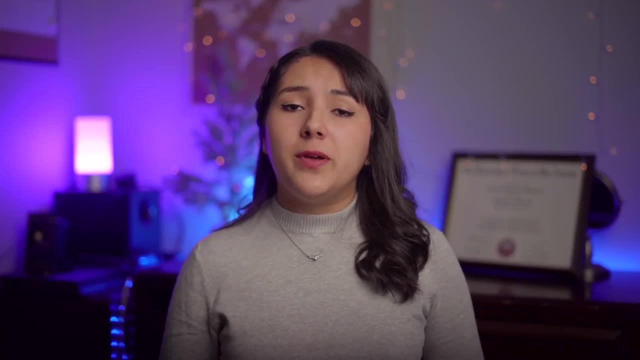 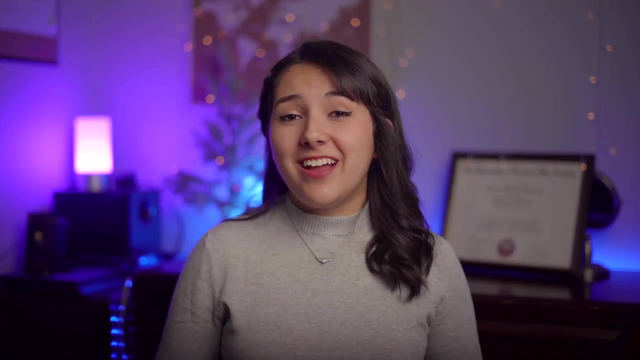 comes to applying for jobs. Another good thing about biomedical engineers is that there is no need to obtain a professional engineer's license. However, this does not mean that biomedical engineers are not high-achieving professionals, as some may even go for a job that is not high-achieving. 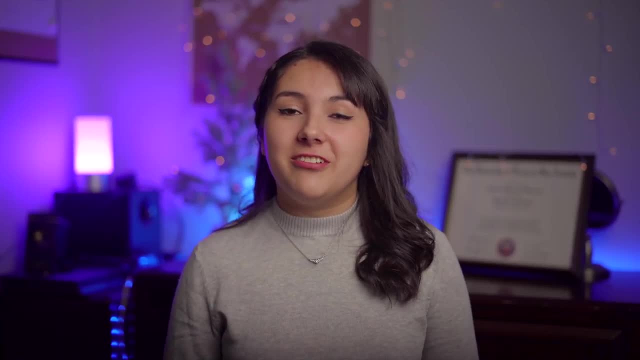 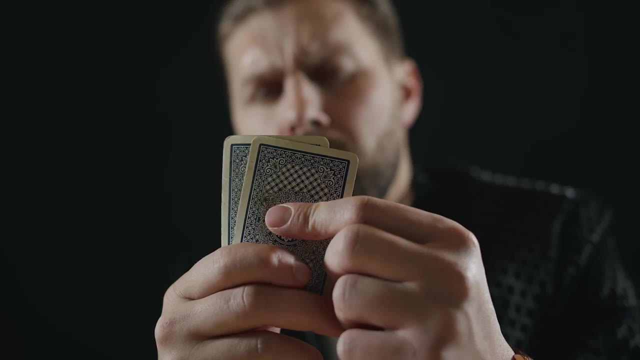 In the end, a BME student will apply for very ambitious degrees like MD-PhD degrees. Number five: you want to learn and use your skills interdisciplinarily. If you haven't heard this before, biomedical engineers are often referred to as the jacks of all trades. This is because 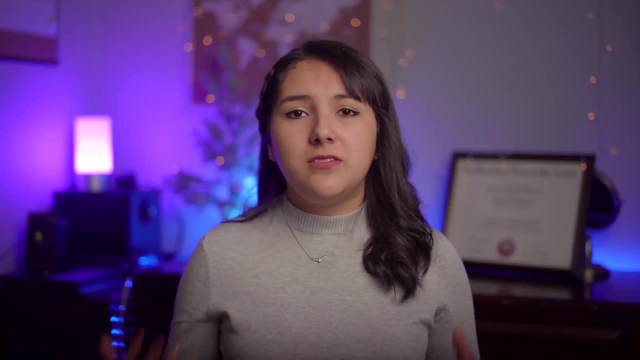 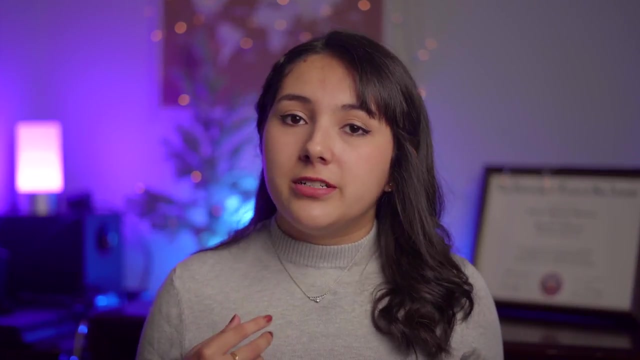 in the BME degree. it subjects you to numerous fields such as mechanics, chemistry, electronics, material science, computer science, biology, engineering and many more. A BME learns to a little bit of everything, which may be good for some, but not for others. I personally think that 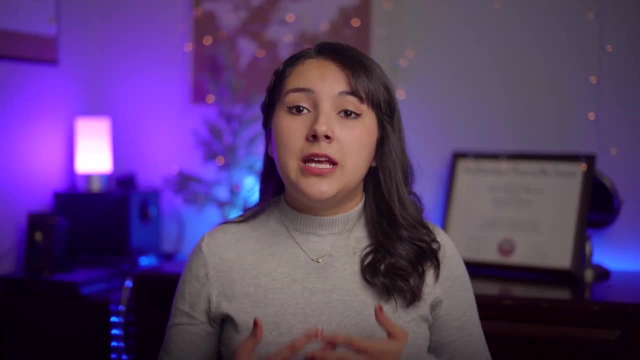 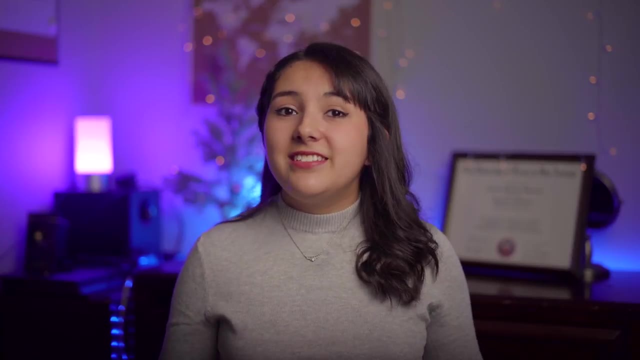 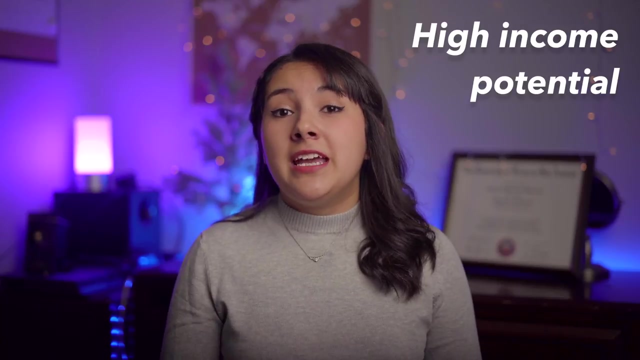 there is beauty in having an interdisciplinary field because, at the end of the day, you will be able to communicate with engineers from different fields, scientists and healthcare professionals. Number six: great income potential. Another reason why you should study BME is because like most engineering degrees, there is great income potential in BME, Although definitely not the best paid engineering. biomedical engineers make more than the average occupation, making around $91,410,, which is only about $3,000 less than the average engineer's salary. of $94,500.. The lowest 10th percentile of biomedical engineers made around $55,280 in 2019.. and the highest 10% made more than $148,210 in the US. Number seven: the opportunity for innovation and entrepreneurship. 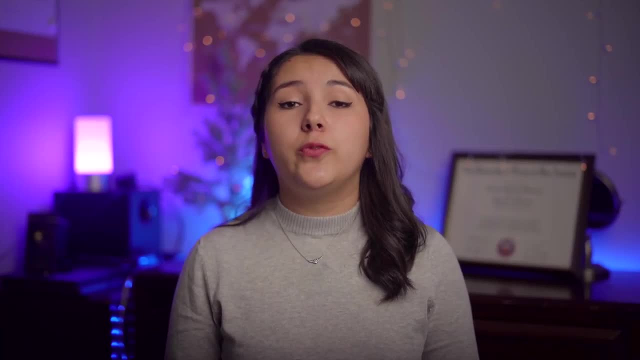 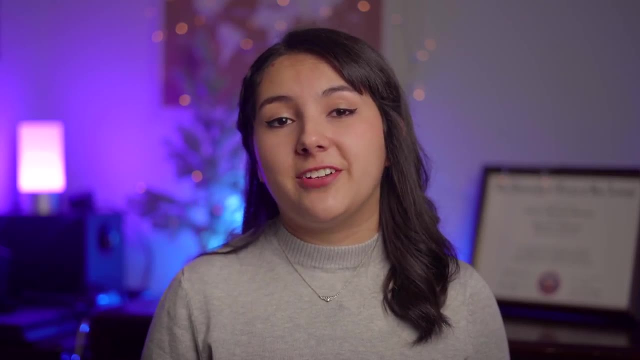 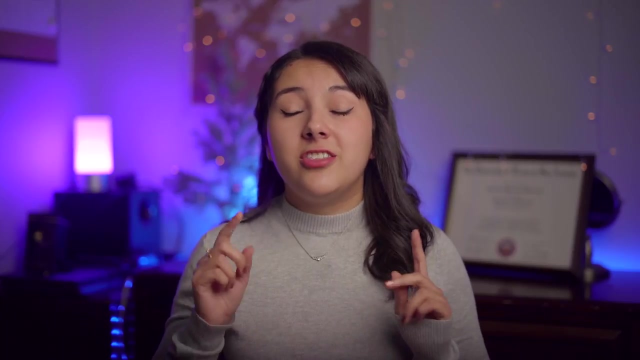 The biomedical engineering field has a lot of potential for young innovators and entrepreneurs. In fact, healthcare is the second most popular startup sector. Biomedical engineers can get exposure to a startup industry as soon as during their college years and are not unlikely to license technologies as students. There's also opportunity for biomedical engineers to work for healthcare technology startups as engineering professionals. Number eight: you want to work in the healthcare technology industry. I know this reason might sound a little obvious, but I just wanted to throw it in here because I have heard of biomedical engineers that are unsatisfied with their career. 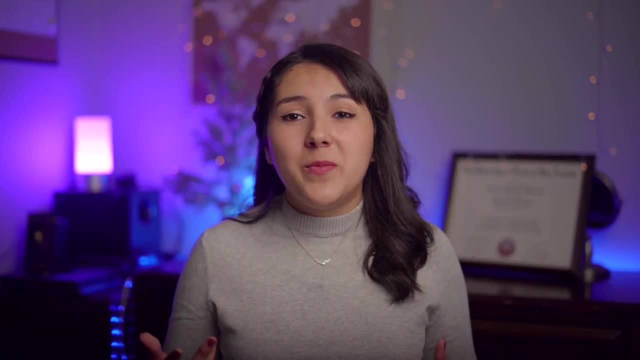 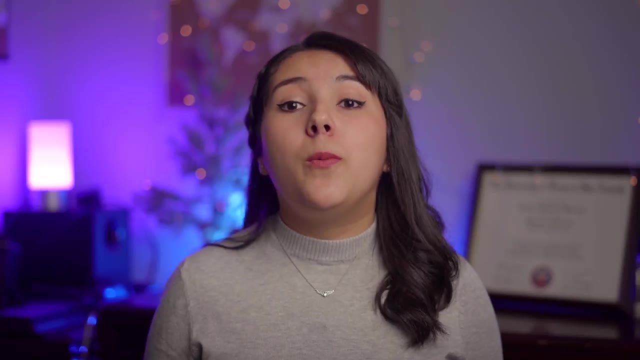 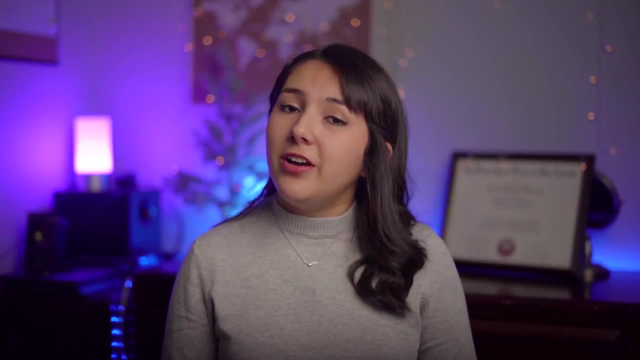 because they feel like they're pigeonholed. They don't want to work in the biomedical technology field. So just take this as a little reminder that as a biomedical engineer, you will more likely be working in the healthcare technology industry. However, some BMEs may venture out into other kinds of industries. 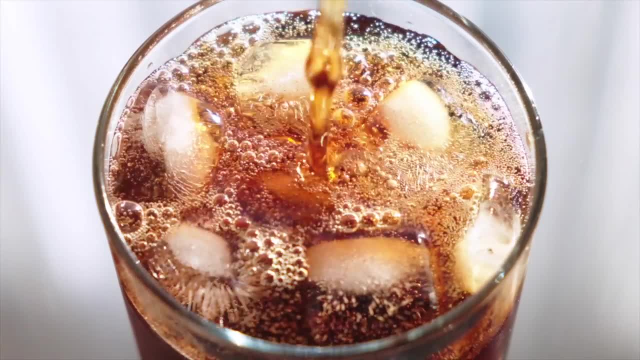 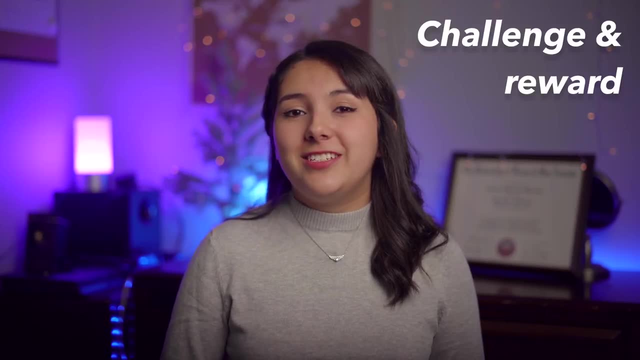 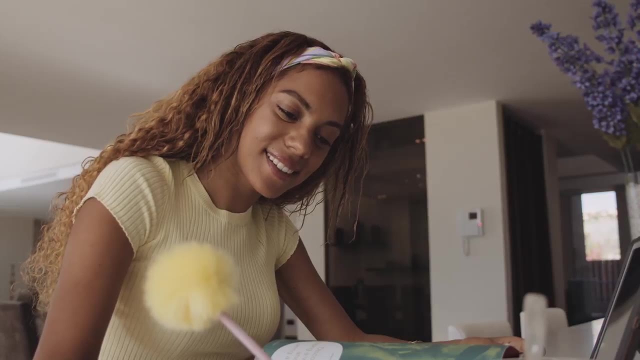 such as regulatory affairs, the food industry and maybe even space exploration. And, last but not least, number nine: you want to be a part of a field that is challenging and rewarding. There is no question about it. There is no question that the coursework of a biomedical engineering degree will be challenging.